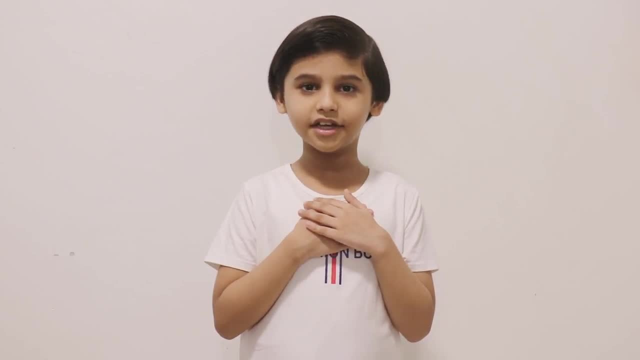 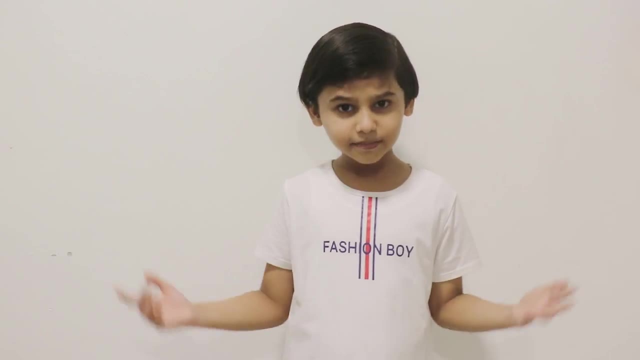 Good day teachers. My name is Tanya Reddy from Year2C. Today I am going to tell you a day in my life. during lockdown, Time is precious- 24 hours make a day, So I am connecting my activities with time. 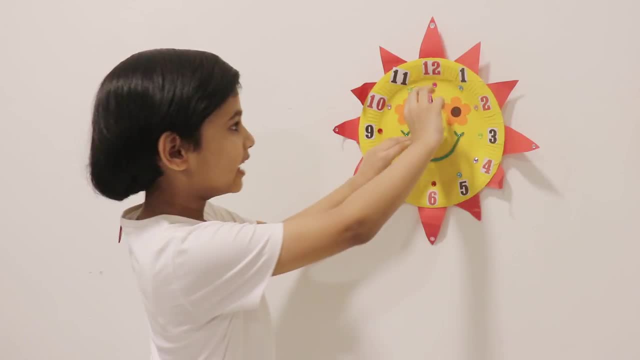 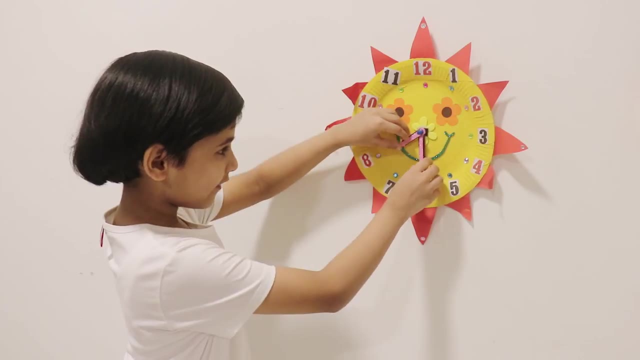 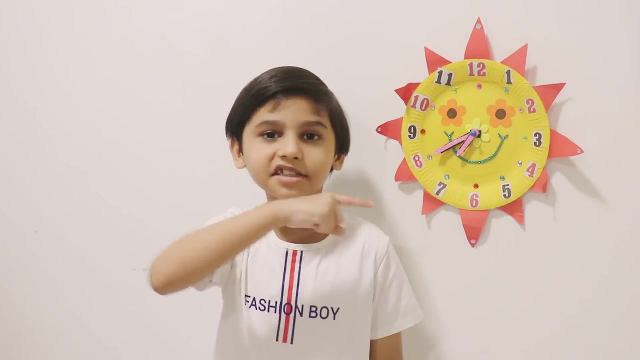 This is a handmade clock. I get up at 7.30 am every day And my day starts there. I will go to use the toilet at 7.35 am. At 7.40 am I will brush my teeth and wash my hands and face. 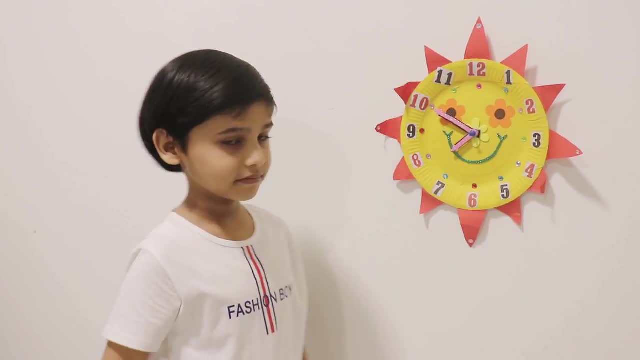 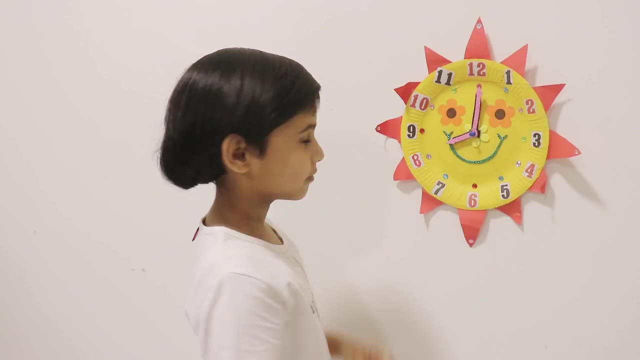 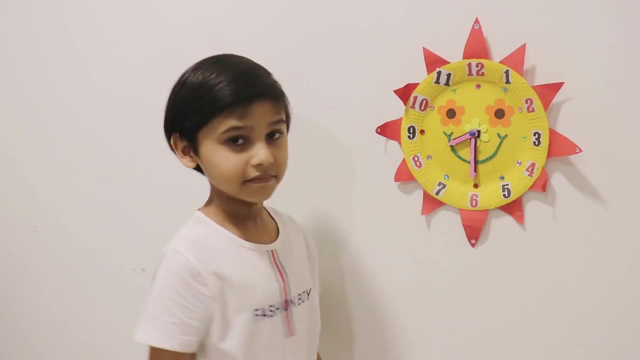 And by 7.50 am I get dressed for my online class. I have my breakfast at 8 o'clock And will attend my online class, which starts at 8.30 am. We get a break at 9.50 am. 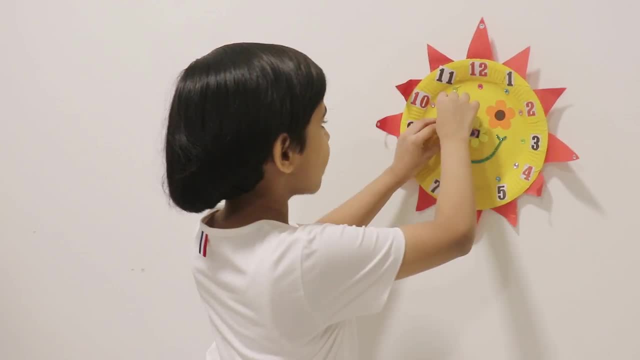 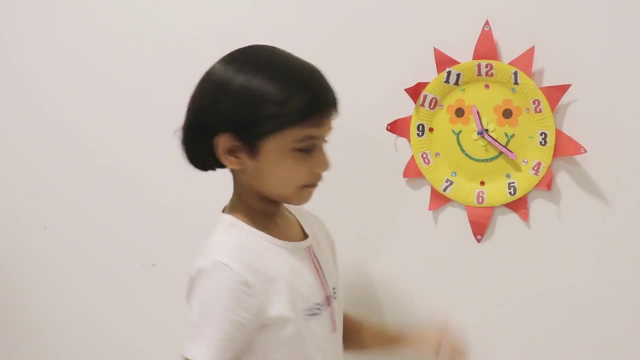 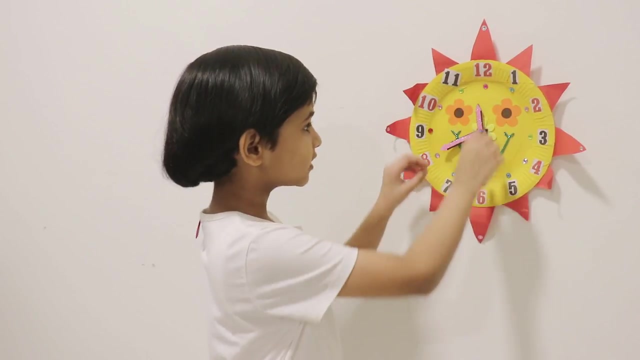 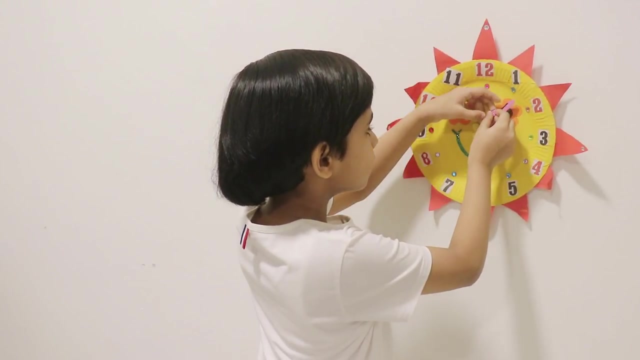 And the class restarts at 10.00 am. The next break is at 11.20 am. The next period starts at 11.40 am. My class ends at 1.00 pm. At 1.10 pm my mummy checks the stream page. 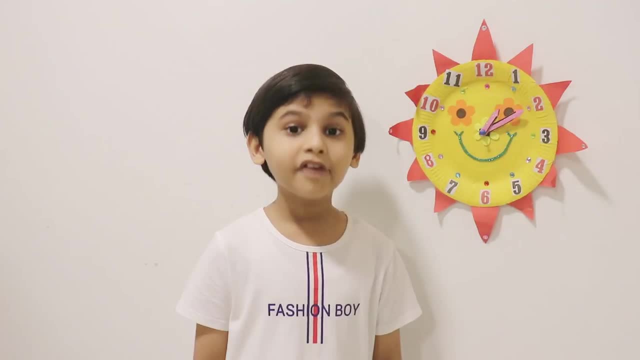 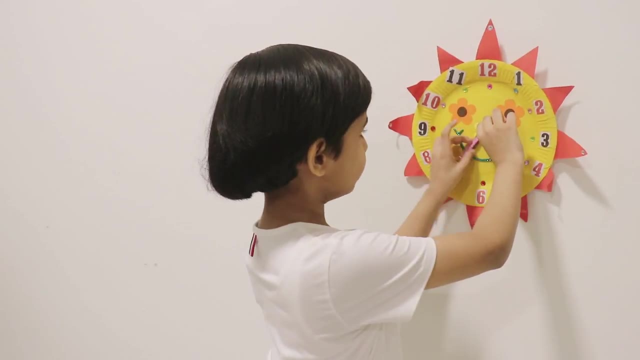 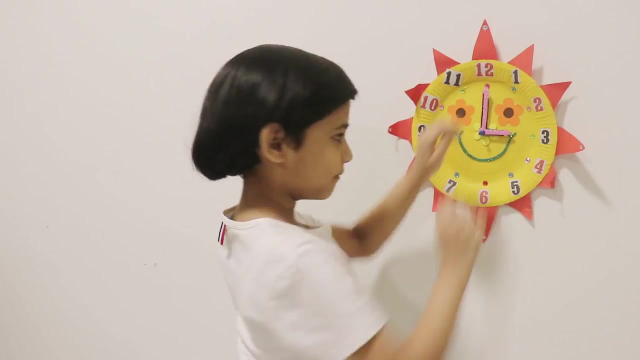 to see what all homework I have to upload At 1.30 pm. we all will have lunch together At 2.00 pm. my sister and I will watch TV till 3.00 pm. Then we will play for half an hour using toys. 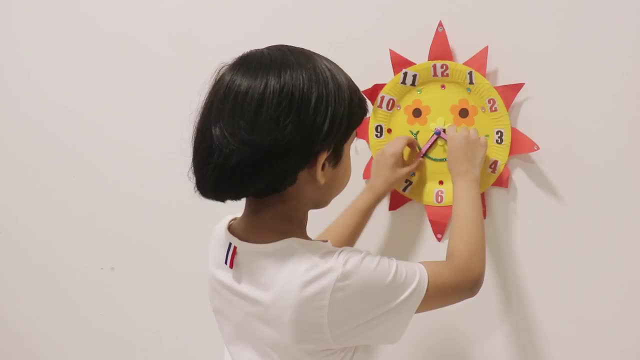 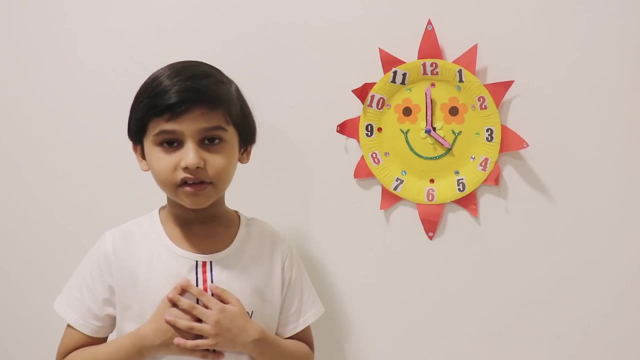 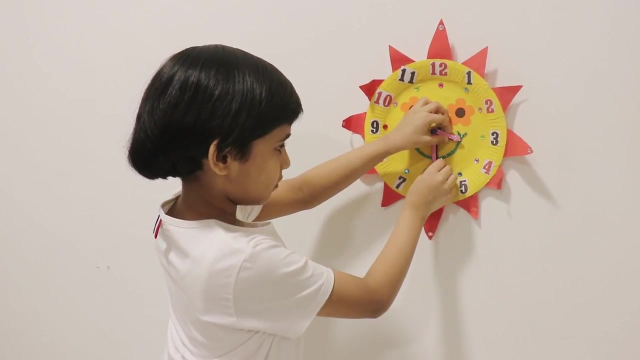 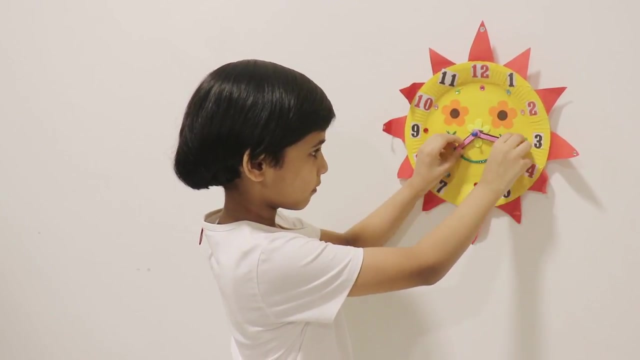 I play the tab for half an hour. At 4.00 pm I will take a bath and get refreshed. At 4.30 pm I start to do my homework. At 7.15 pm I will start studying. 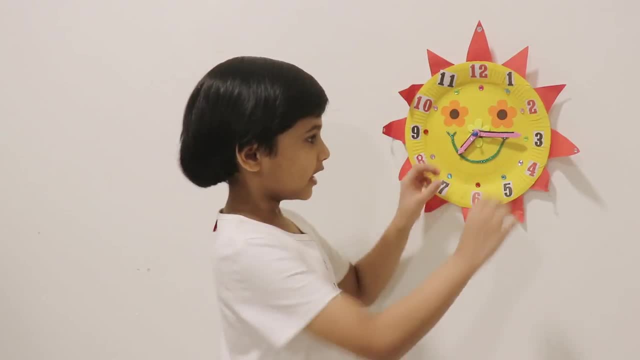 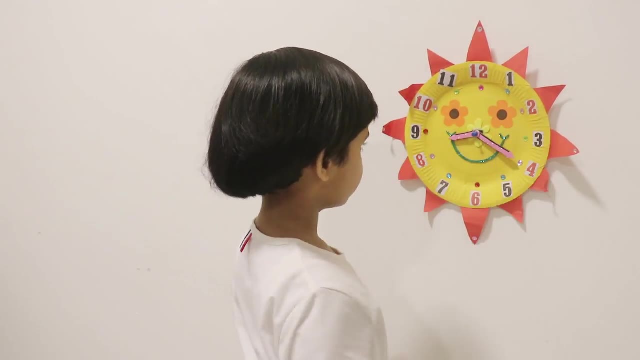 I will study if there is an assessment on the next day. At 8.20 pm I will study if there is an assessment on the next day, And at 8.30 pm I will have dinner. If no other work to do, we will watch TV again for one hour.